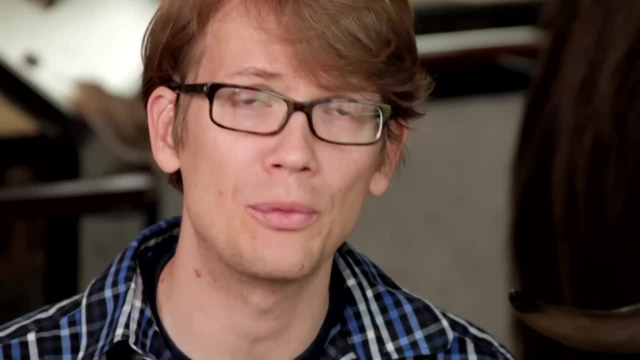 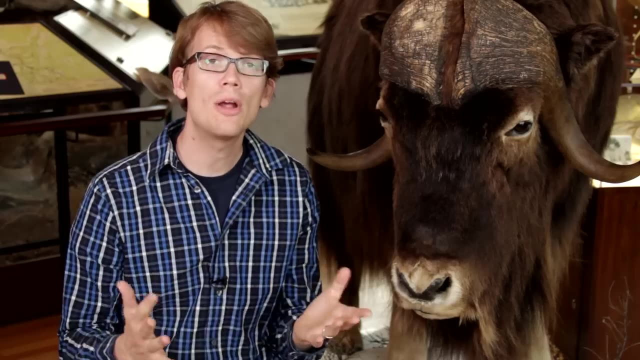 In the end, the effect of predator-prey interaction is an evolutionary arms race that results in the mind-boggling amount of diversity we see in any ecosystem, from the Northern Rockies all the way to the African savannah. This arms race is known as coevolution. 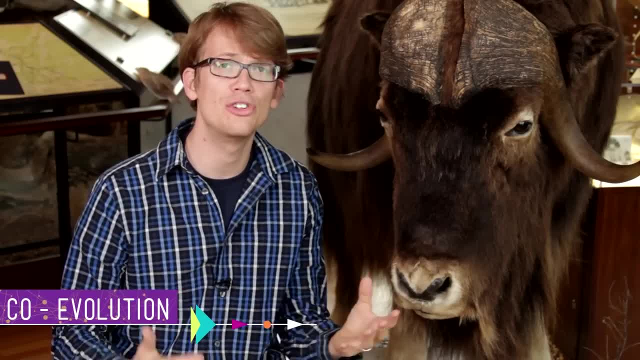 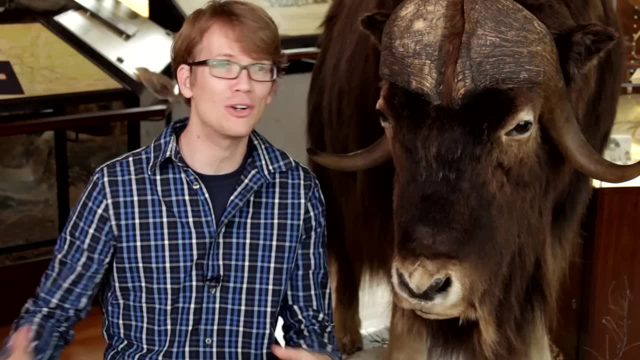 the process by which the interactions between two species affect the evolutionary development of both. It's been going on since the Cambrian explosion more than half a billion years ago and it will continue, spawning new bursts of diversity long after we humans have eaten ourselves into extinction. 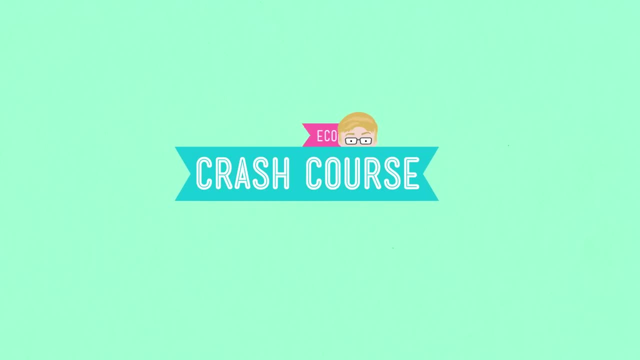 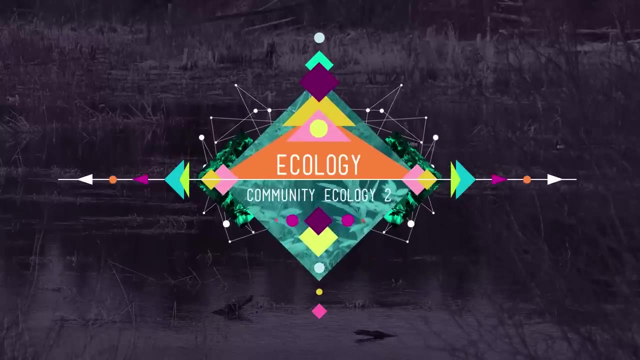 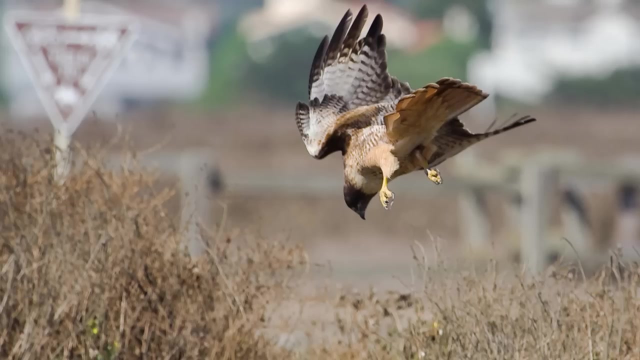 And maybe we'll end up in a place like this. We tend to think of predation in terms of animals- Lions hunting zebras, wolves killing sheep, hawks eating mice- But predation is much more than carnivores doing their thing. It applies to any number of interactions where one type of organism kills another for its energy. This is an important thing to note because a lot of ecology comes down to the flow of energy through nature, And every living thing needs energy to meet its twin evolutionary goals of staying alive and making lots of babies. Predators kill because they're hungry, but they're hungry because they need energy to survive and reproduce For prey. these interactions are especially high stakes, obviously because nothing quite quashes your reproductive chances like being dead. But almost all energy on Earth starts with plants, so consider bison eating grass. 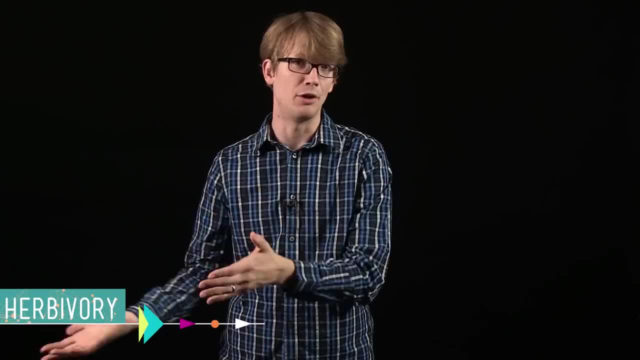 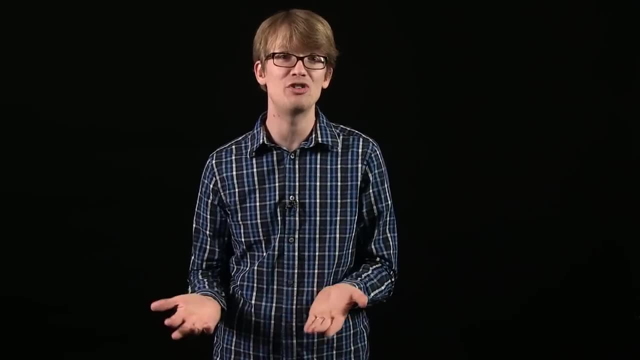 That's a type of predation called herbivory, where an organism eats plants or algae to capture their energy. It may not really seem like predation to you, but bison eating grass, manatees eating seaweed and sea urchins munching on algae. 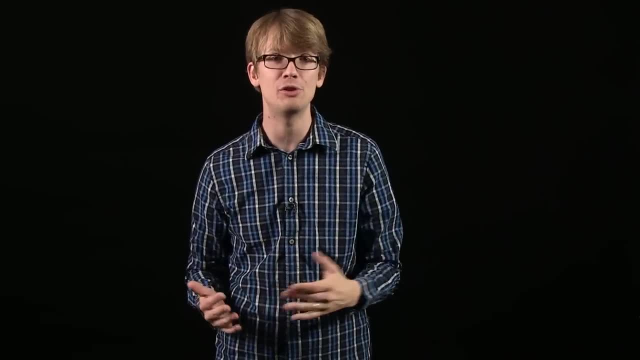 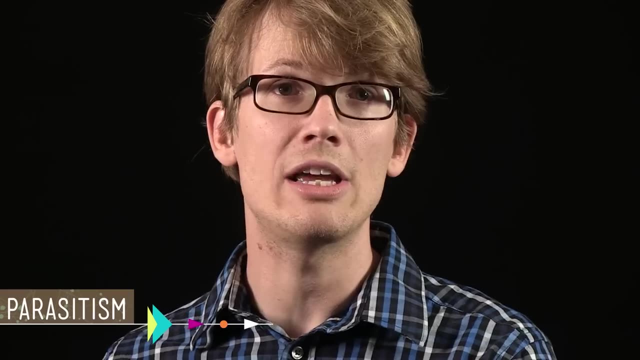 are all examples of organisms eating other organisms to ingest the energy of the sun. There's also parasitism, another form of predation in which organisms derive energy from a host, usually harming it and sometimes killing it in the process. Hairworms, for example, devour the insides of grasshoppers. 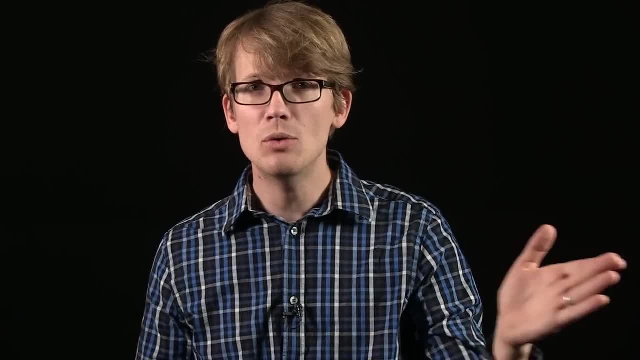 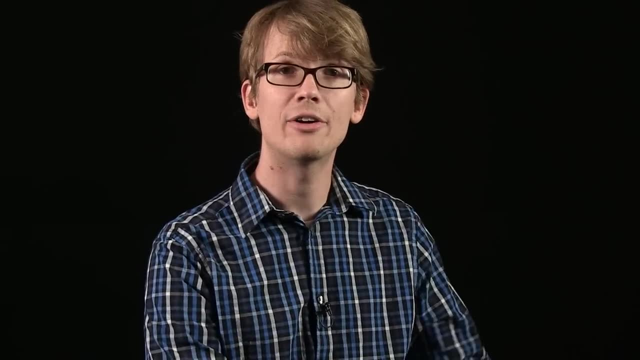 and then brainwash them to make suicidal leaps into water. How exactly the water-born worm finds its way into a grasshopper is a mystery, though larvae carried by mosquitoes is a likely route. Once inside the grasshopper, the worm eats everything non-essential to its host. 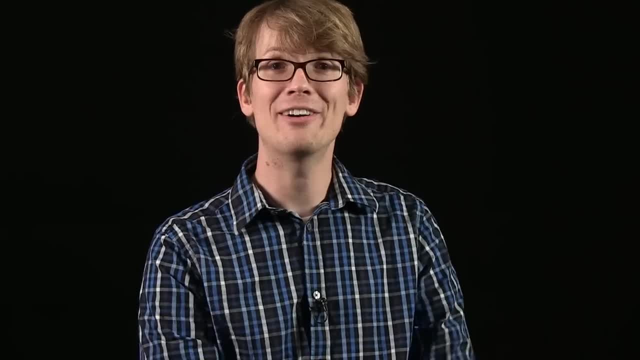 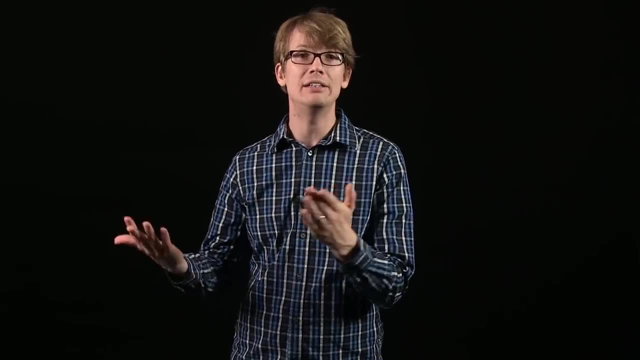 as it grows several times the length of its host's body. When only the grasshopper's head and legs remain, the hairworm is ready to reproduce, And that's when the brainwashing begins. See, hairworms breed in water, but grasshoppers can't swim. 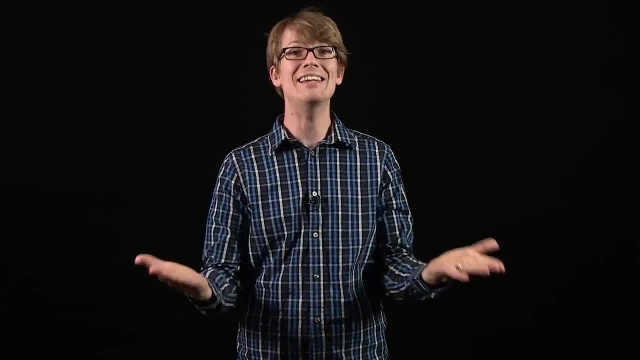 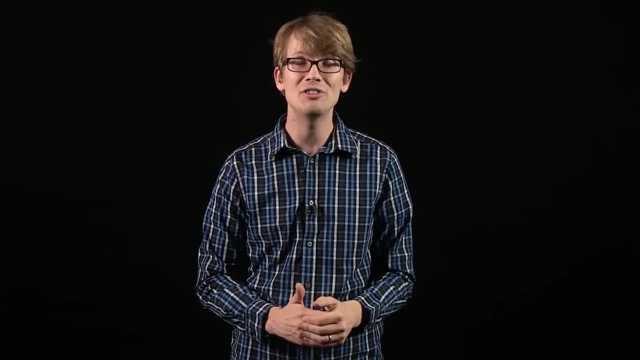 So hairworms pump their hosts full of chemicals that prompt an inescapable urge to leap into a body of water. Once the grasshopper makes the leap, the hairworm is free to burrow out of the host and find a mate. 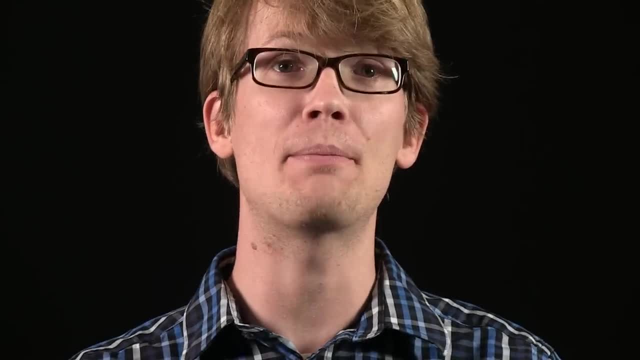 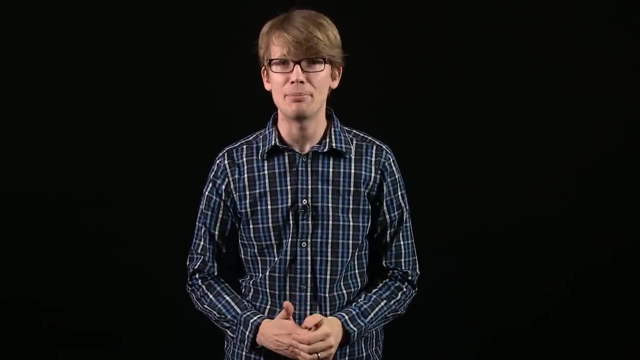 Ew Yeah, chasing and eating a gazelle is one thing, but turning your prey into like a suicidal zombie- that, my friends, is predation. So clearly, predator and prey- both have millions of years of tricks up their sleeves. 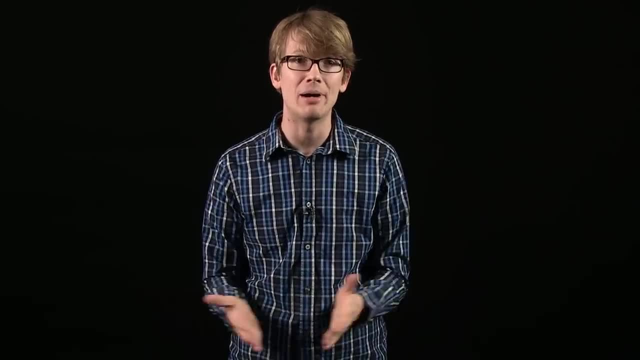 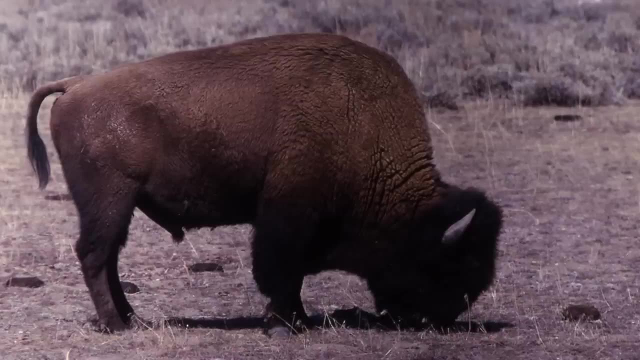 or stored in their DNA, because everyone's ultimately playing by the same set of evolutionary rules. Whether lion or zebra, grasshopper or hairworm or bison or grass, gaining energy while not being eaten is a prerequisite to reproductive success. 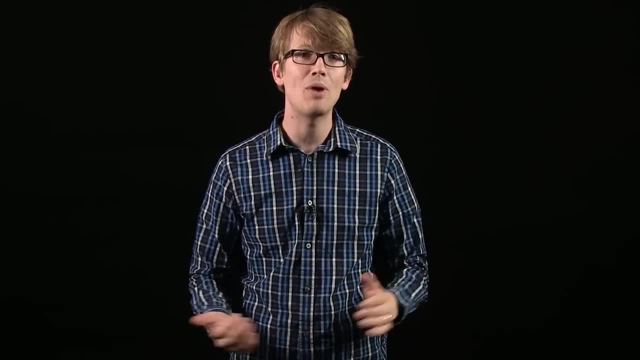 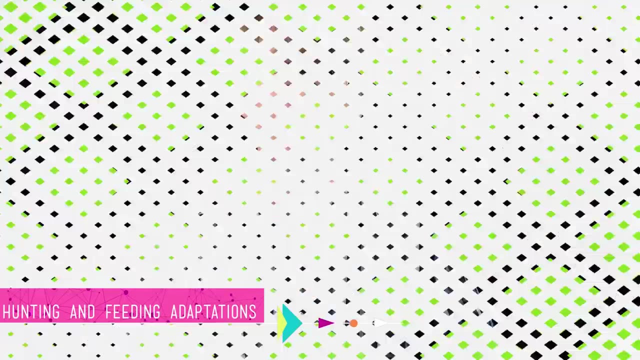 But the need to survive constantly forces predator and prey to adapt weapons and defense in a never-ending evolutionary arms race. On the predator side, hunting and feeding adaptations are obvious and familiar: A wolf's keen sense of smell, flesh-ripping teeth. 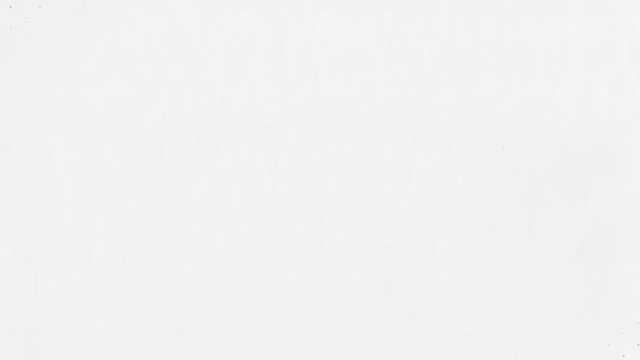 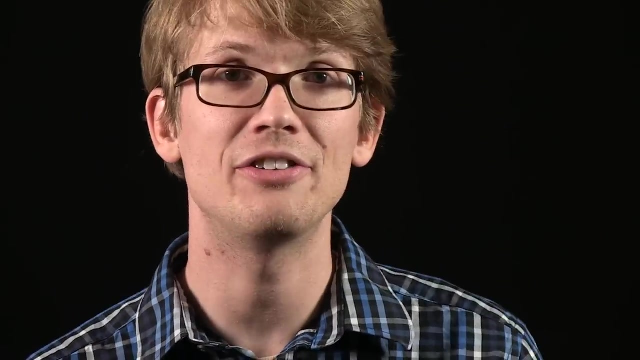 and an eagle's sharp eyes and prey-gripping talons. Other creatures like rattlesnakes use heat-sensing organs to seek out small rodents and toxic venom to strike them dead. But this is where coevolution takes the stage. 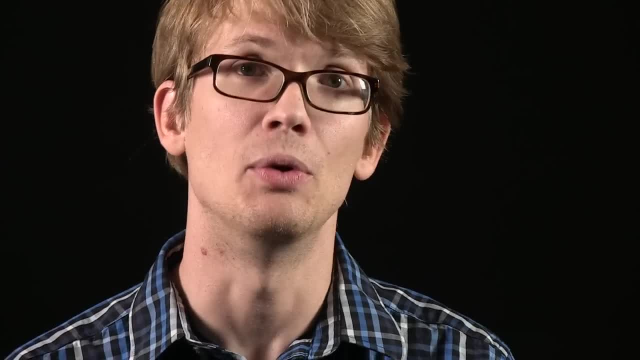 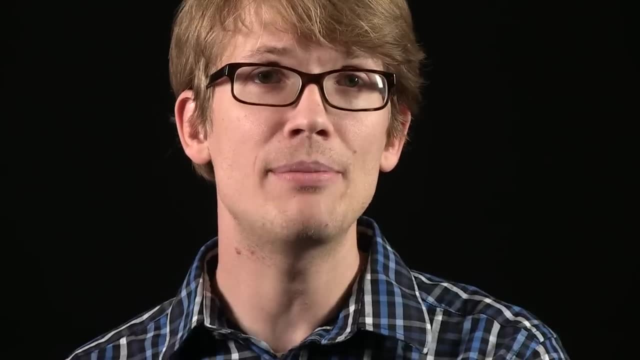 to give the prey a stake in the evolutionary arms race too, Since, being caught by a bird, it's hard to tell if it's a predator or not. A predator is kind of terrible for anything that hopes to spread its genes. Species have adapted to all sorts of ways to avoid getting killed. 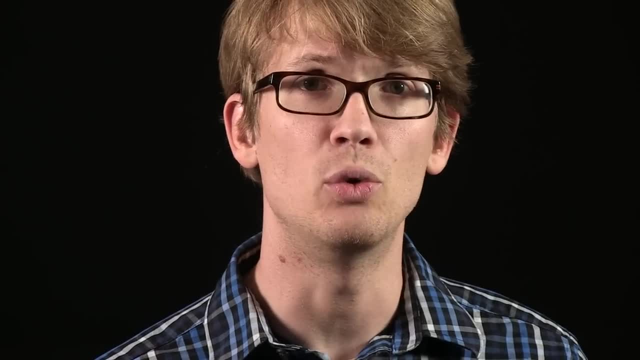 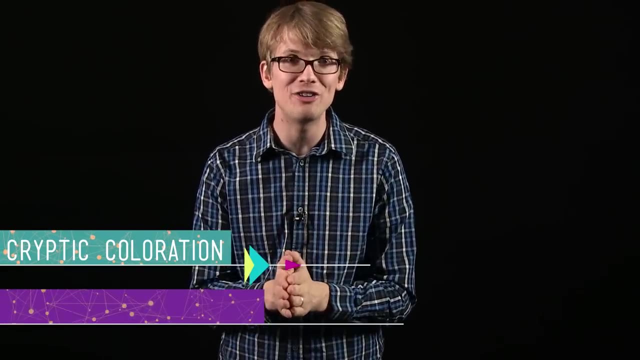 These can be broken up by what kinds of predatory behavior these adaptations are designed to avoid, Namely detection, capture and handling. To avoid detection, some prey adapt cryptic coloration, which we better know as camouflage, to help a species blend into the background. 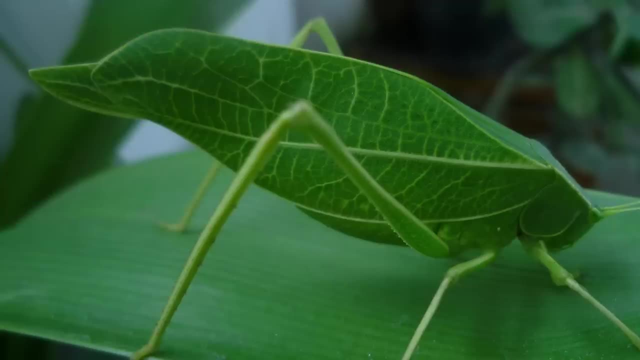 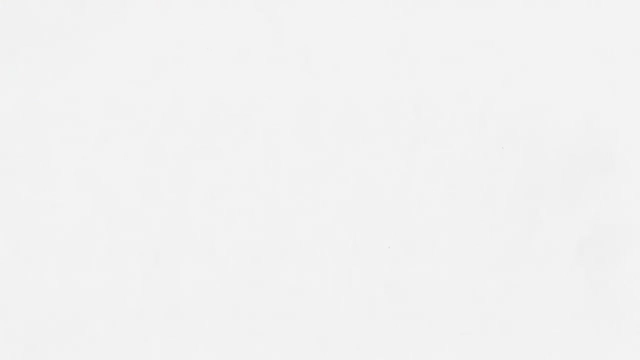 Stick insects that have adapted to look like sticks, leaf insects that look like leaves, snowshoe hares that turn white in the winter to blend in with the snow and brown in the summer to blend in with the rain. The grasses are all good examples. 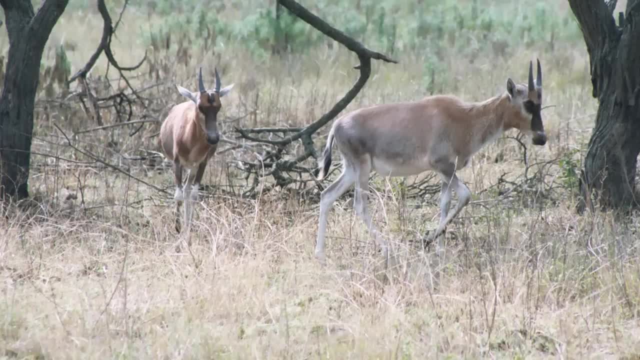 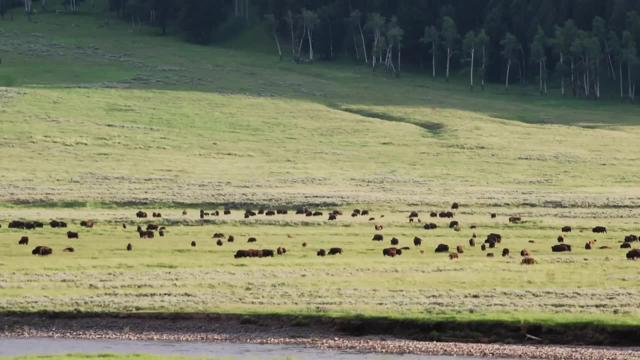 Avoiding capture is at times pretty straightforward. Antelope, for example, flee predators with great leaping speed. Others find safety in numbers, such as a bison forming giant herds or herring grouping in schools. This kind of grouping certainly doesn't protect the prey from being detected. 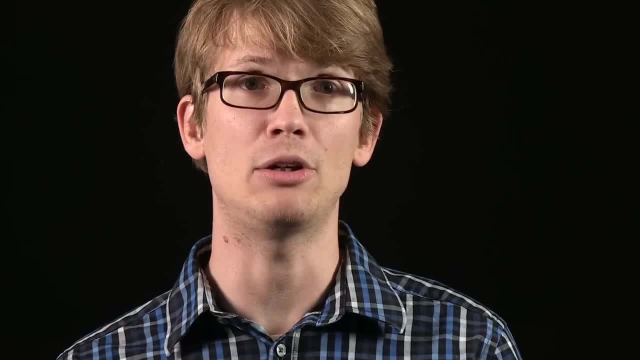 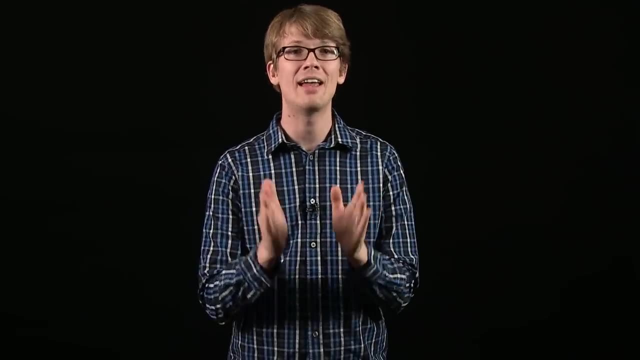 but it greatly reduces chances that any individual will get picked off by a predator, especially fit members of the group in the middle of the pack. And finally, some of the coolest and most familiar adaptations are those that prevent handling. Plants are experts at these. 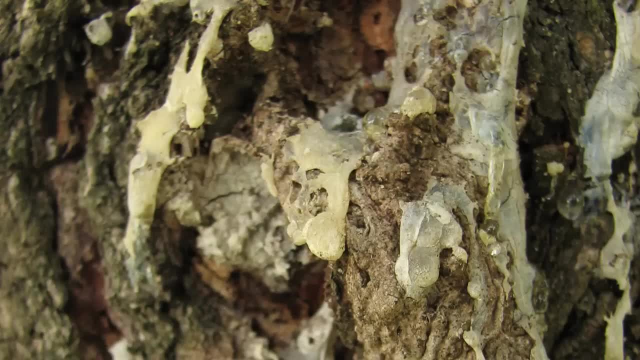 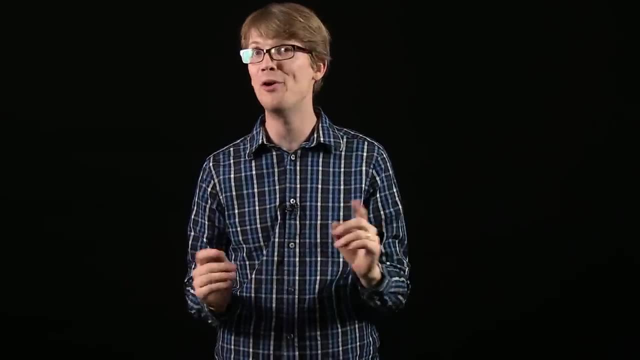 Think of a rose's thorns, a tree sap that traps insects through the branches of an African acacia tree. They're most thorny within the range of tree-munching giraffes, but above, where the long necks reach, there aren't as many thorns. 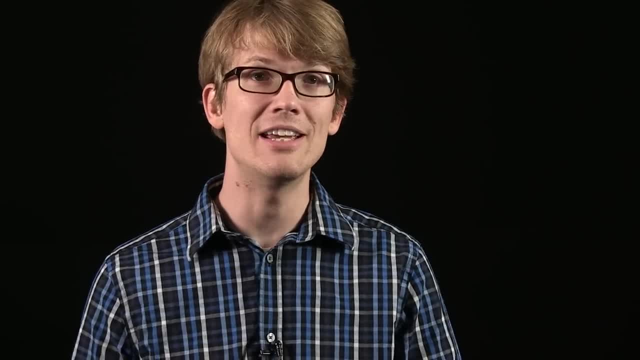 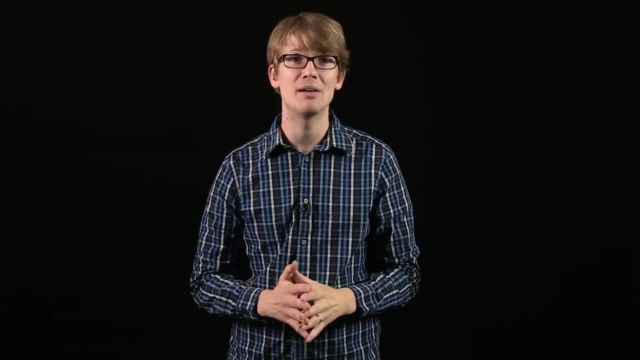 Other plants also produce chemical weapons, such as the tobacco plants, nicotine and the tannins produced by many plants like grape vines to fend off foragers. But things get really weird when you see what animals do with this bag of chemical tricks, because often these critters not only have wicked toxic cocktails to defend themselves. 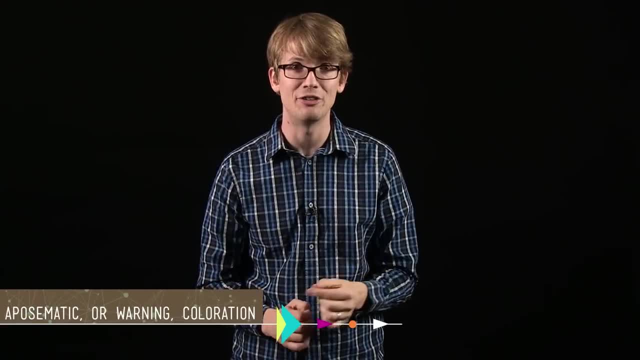 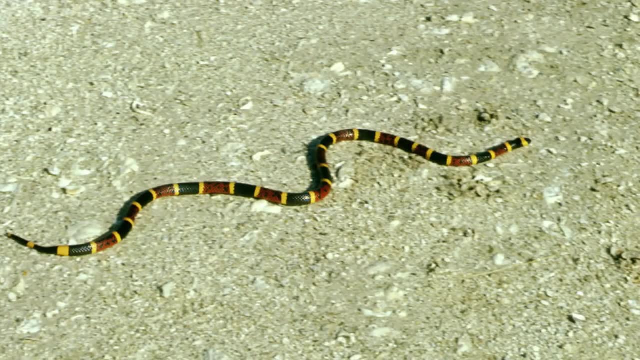 many have also evolved aposematic or warning coloration. The bright contrasting colors, such as yellow and black splotches of the fire salamander or the red, yellow and black bands of the coral snake, make it clear to predators that eating them would be a serious mistake. 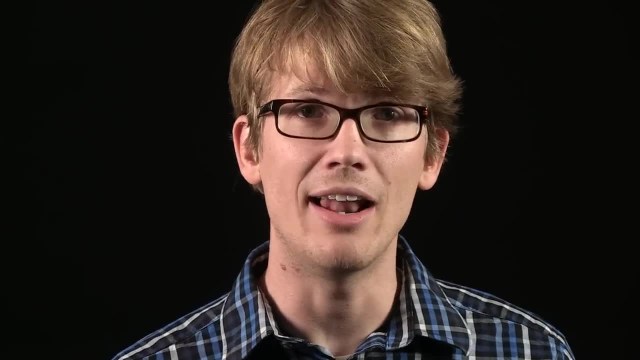 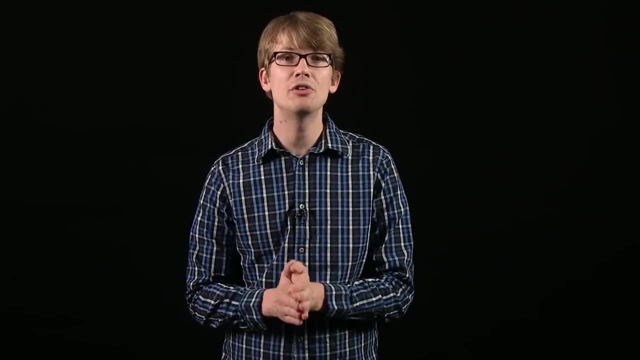 And when you think of it, nature is full of species that are black and yellow in color or red and black. We tend to avoid them at all costs. We're smart that way, and so are most other predators. This, of course, is no coincidence. 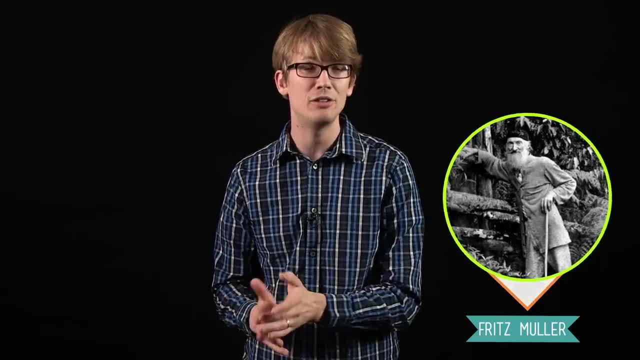 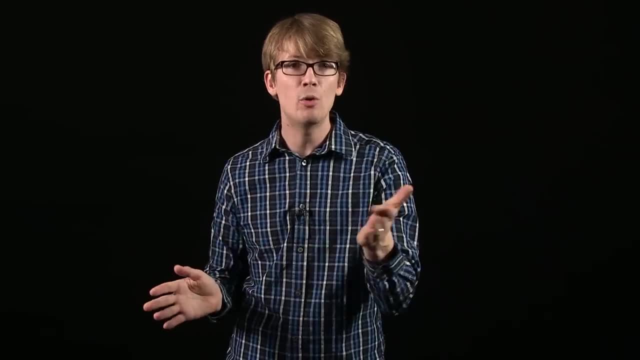 As German naturalist Fritz Müller noted in the 1870s, unpalatable species such as cuckoo, bees, yellow jackets- actually almost every kind of bee and wasp- resemble each other with different colors and patterns. He figured out that the more unpalatable prey there are. 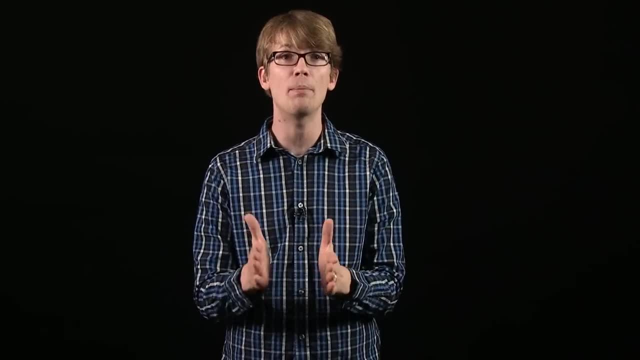 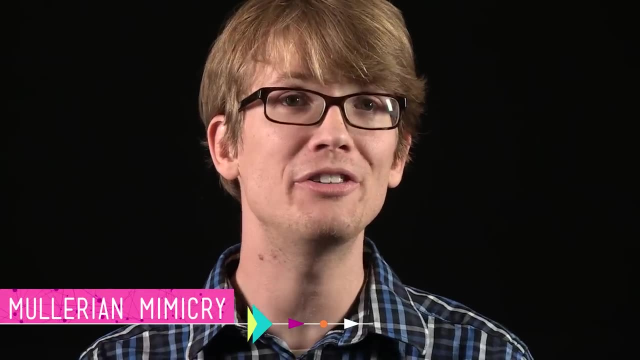 that use the same color patterns, the more likely predators are to avoid all prey with that appearance. in general, This defense technique is today known as Müllerian mimicry, But it turns out unsurprisingly. some critters that look dangerous are getting the last laugh. because many of them would actually be quite tasty to any predator. They just trick everyone by copying the looks of the truly dangerous species. This technique is called Batesian mimicry, and to explain it to you I'm gonna need to sit down. 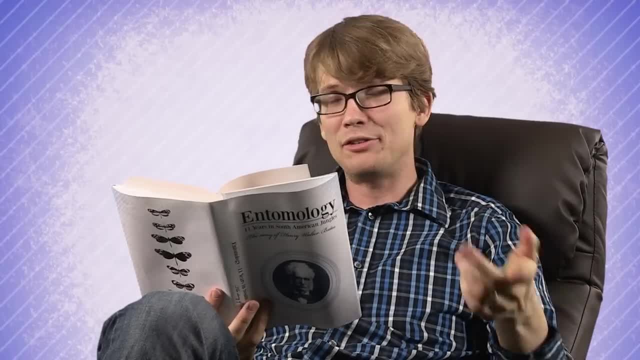 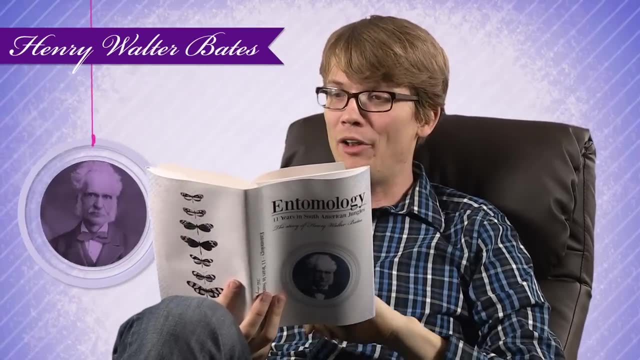 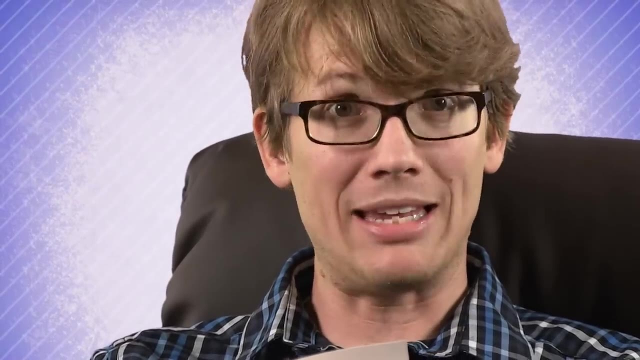 I'll give you one guess to figure out who first described Batesian mimicry. That's right, it was Bates. More specifically, it was Henry Walter Bates, a 19th century British naturalist and explorer. Bates was born in 1825 to a middle-class family that paid the bills by making hosiery. 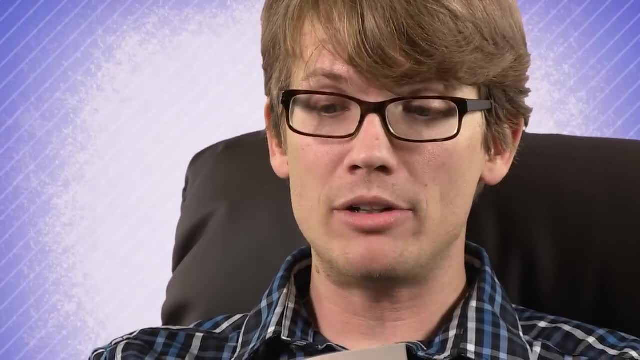 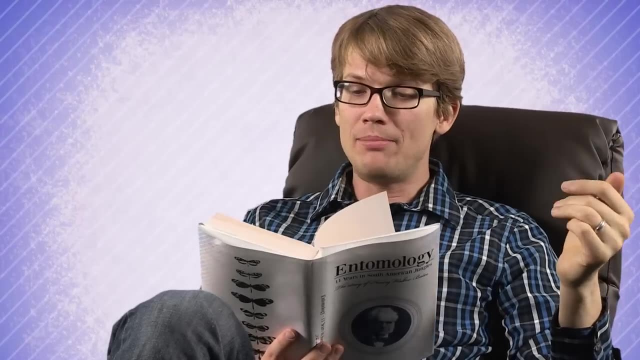 He spent most of his spare time reading, often about bugs, and by the young age of 18, he was a budding entomologist, with a publication on beetles already, to his credit. It was a few years later that he met the famed entomologist. 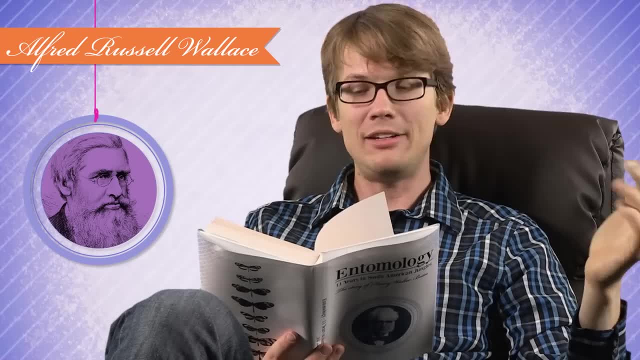 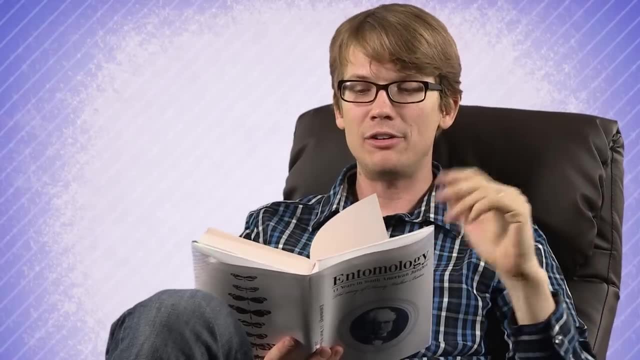 Alfred Russell Wallace. The two hit it off and Wallace, in 1847, proposed to take a trip to South America to collect insects. They would finance their travels by sending collected specimens back to England for sale to museums and private collectors. The pair set sail the following year and after four years in the field, 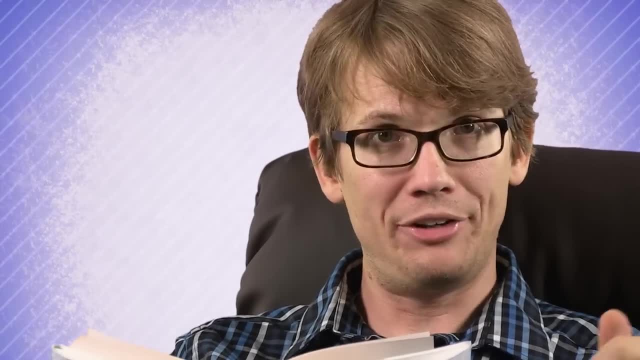 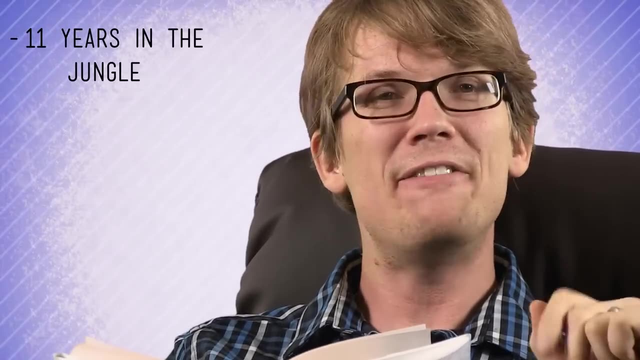 Wallace moved on, But Bates, apparently not wanting to get into the hosiery business, stayed behind, spending the next 11 years in the jungle. All told, he collected nearly 15,000 species, about 8,000 of them. 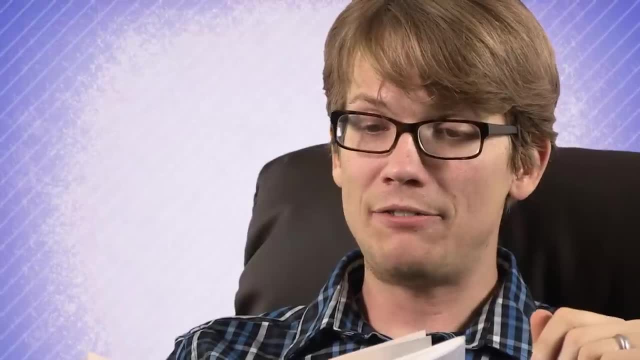 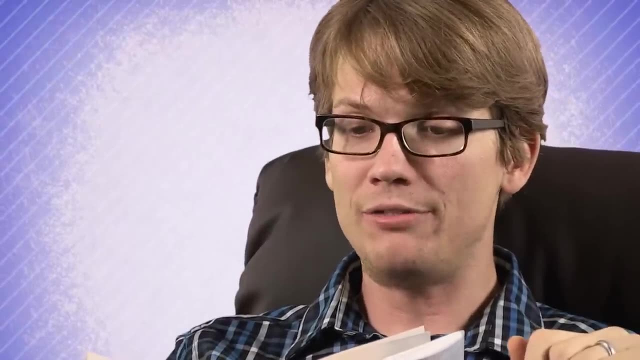 Just a few months after Bates arrived home, in 1859, Darwin published his On the Origin of Species. Bates read it and figured he could contribute evidence to support the new theory of natural selection from his insect collection. Two years later he presented a paper that showed how different species of butterfly 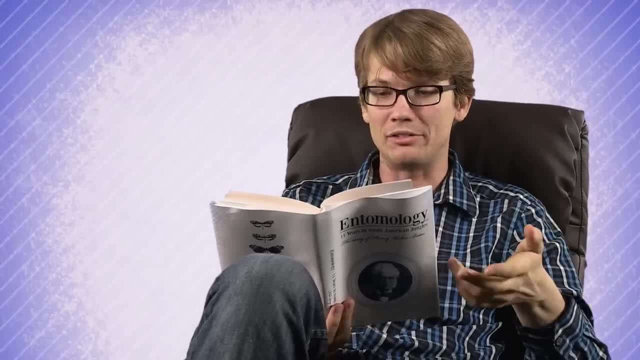 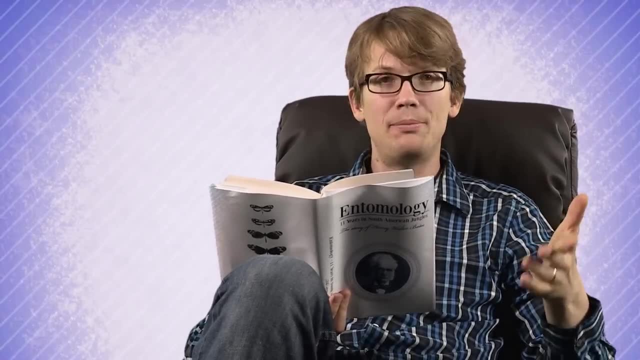 developed nearly identical color patterns on their wings. For example, butterflies called Heliconianae, which were slow-moving and abundant but toxic, were nearly identical to Pieridae, which were more rare but harmless. Bates concluded that natural selection had driven the harmless butterflies. 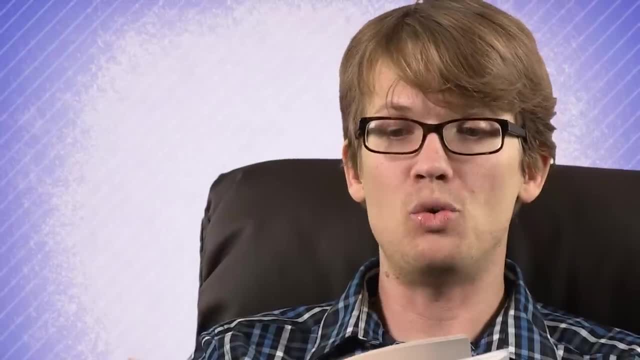 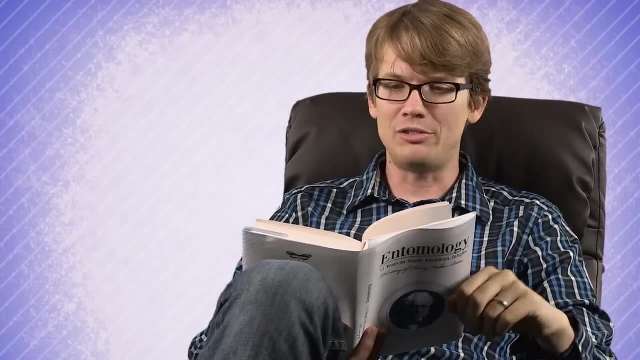 to mimic the patterns on the harmful butterflies for their individual bids to survive predation by birds. The discovery helped launch Bates' career and reputation, and he went on to recount his adventures and other discoveries in a book: The Naturalist on the River, Amazon. 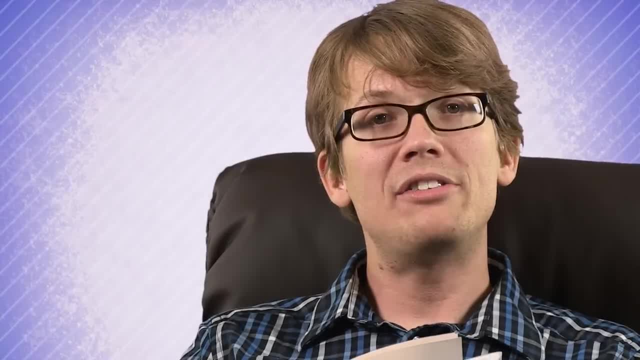 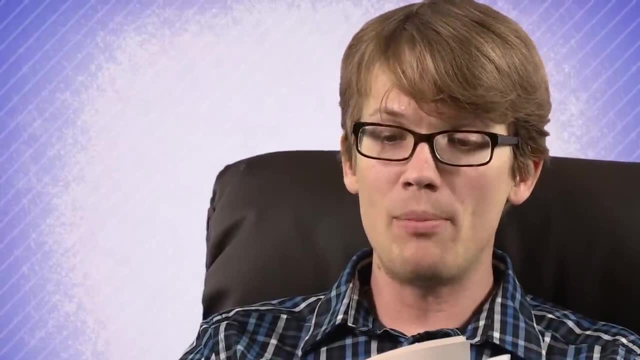 and later took a job as secretary to the Royal Geographic Society. Though Bates died in 1892, the concept of Batesian mimicry continues to fascinate scientists today. Why, for example, are so many mimics not perfect imitations of their more dangerous counterparts? 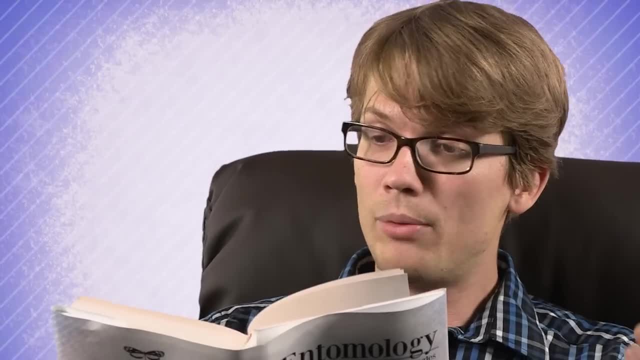 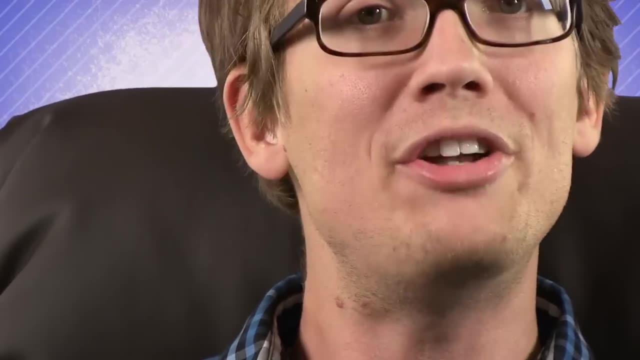 Is it because perfect imitation isn't necessary to do the job, or because mimics lack the genes necessary to perfectly resemble their poisonous counterparts? Perhaps budding entomologists armed with 21st century tools will finally unlock the answers. But don't think that prey are the only crafty mimics out there. 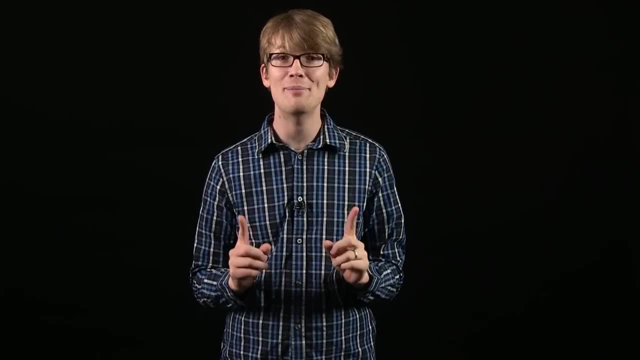 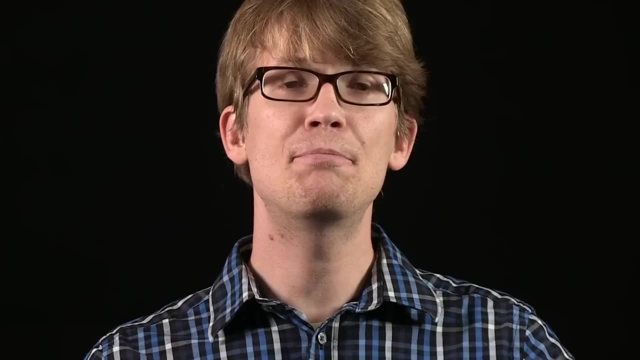 In the arms race, some predators have learned how to win food through imitation as well. You've heard me talk about snapping turtles with tongues that resemble wiggling worms to lure fish, and don't get me started about anglerfish. If predation teaches us anything, it's that nothing lasts forever. 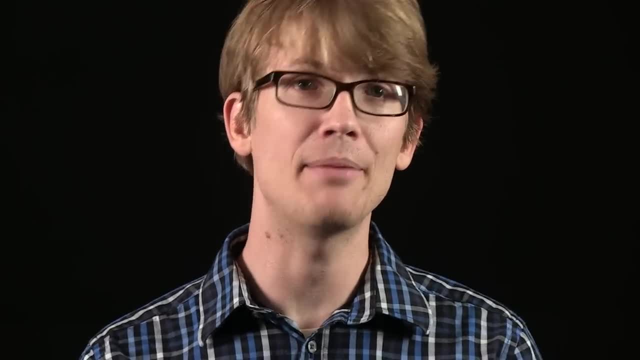 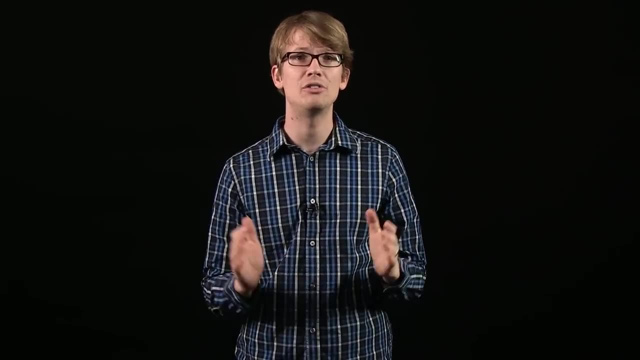 not just for prey but for every living thing, because the interaction between predator and prey keeps driving evolutionary change. But the communities themselves that we've been talking about for the last two weeks don't stay the same either. of course, New tenants are always moving into a habitat.